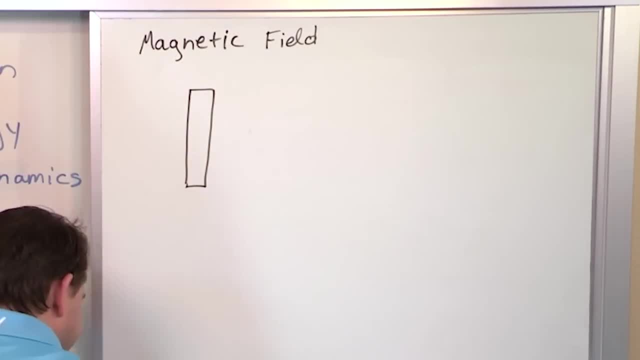 have a bar magnet here right North pole, south pole. remember all that stuff when you were a kid. It turns out that we in physics talk about this invisible field that surrounds it. We can't see it, We can't really touch it, but we know it's there because it can make, it can influence the. 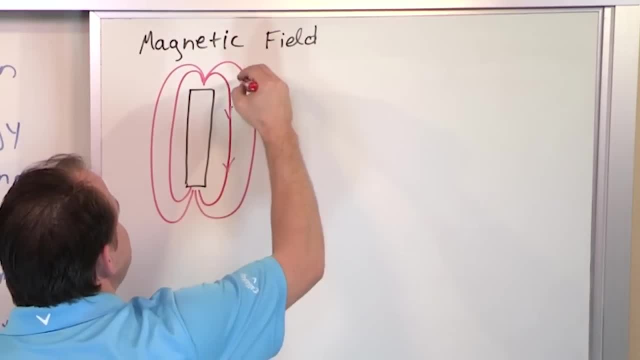 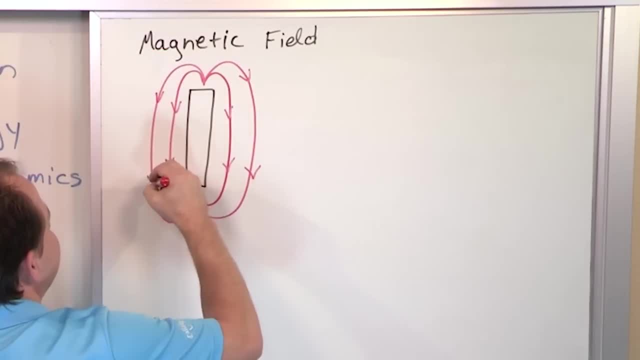 call a magnetic field, lines which are kind of invisible, lines of kind of a force- you can think of it that way- that surround this guy And then we have, analogously to this, a magnetic field, I told you, an electric field. they're kind of like peanut butter and jelly. So if this is the peanut 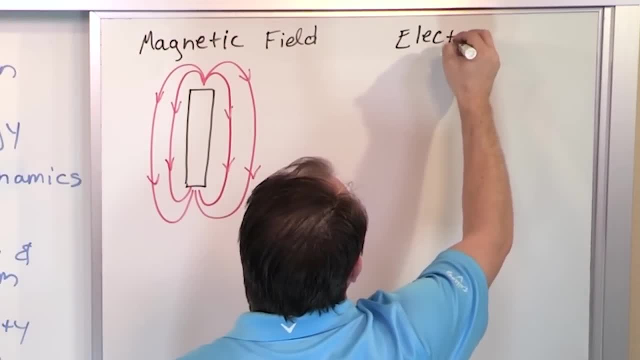 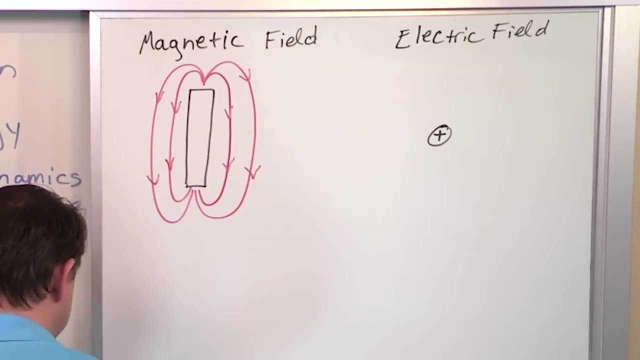 butter. the jelly is called the electric field. So if we have, for instance, a proton, there's a proton or neutron that goes to the other direction with a positive charge. There There's an invisible field that we say surrounds this guy, But it doesn't form these closed loops like this. 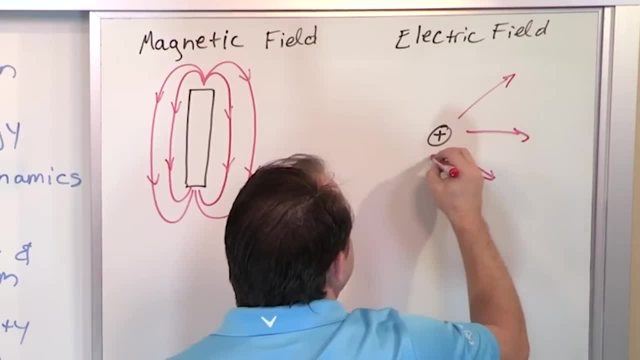 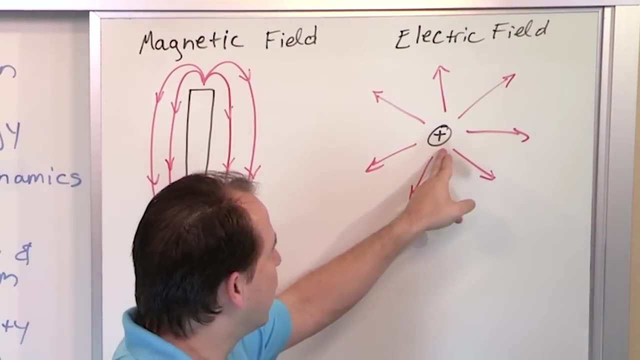 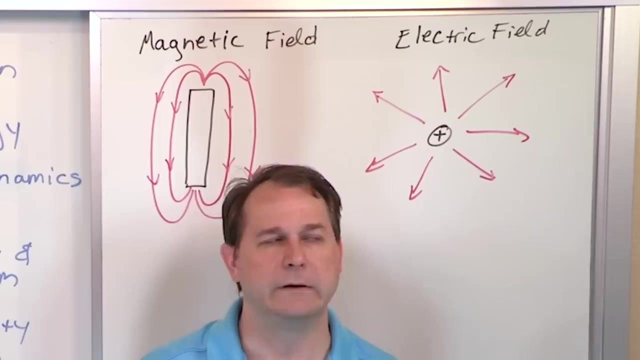 It forms kind of these radial kind of arrows that kind of emanate from the charged particle. So it works for protons and it also works for any charged particle. So there's an electric field that surrounds an electron also, but it goes the other direction. And so what we basically say is: you can. 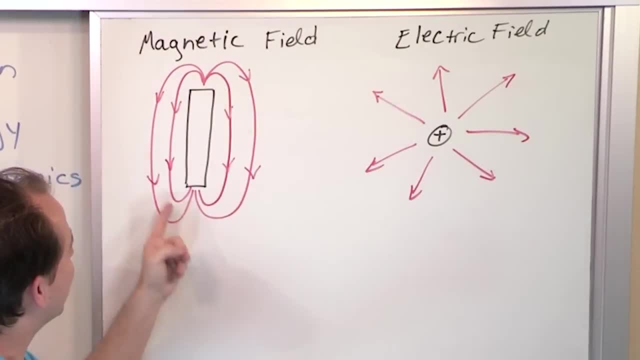 see there's some similarities between the two, but there's a difference in that. So, as we go from similarities here, but there's obvious differences- I mean, these guys form loops, these guys don't form loops, And the other main difference is sort of like how they were. 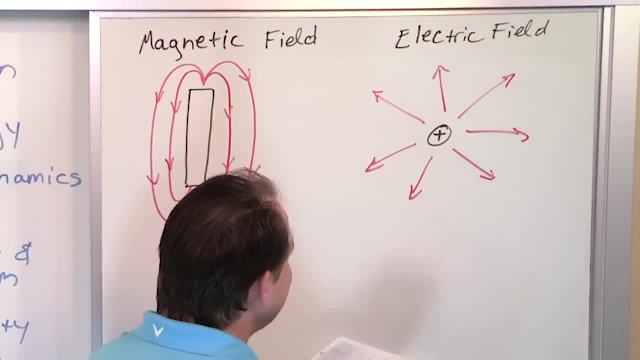 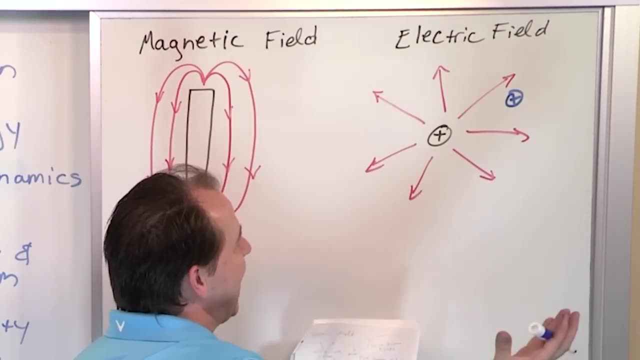 discovered. to begin with, If I were to take another proton and stick it inside this electric field right here, like this is a test particle, what's going to happen? It turns out that this electric field is going to push on this charged particle and it's going to push with a force F. 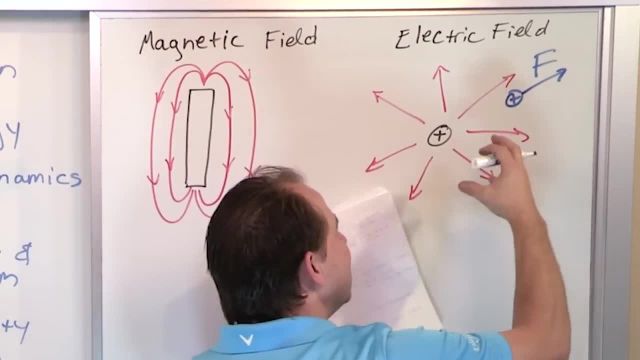 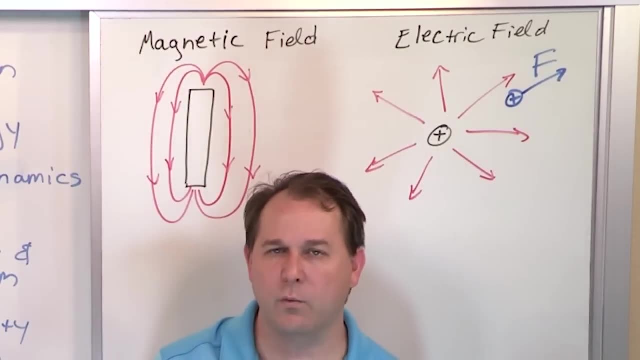 and it's going to push it directly away from this guy. Remember, like charges repel and opposites attract. So we say in physics is that, instead of just saying like charges repel, what we say is that this charge generates an electric field and that electric field is what pushes on the 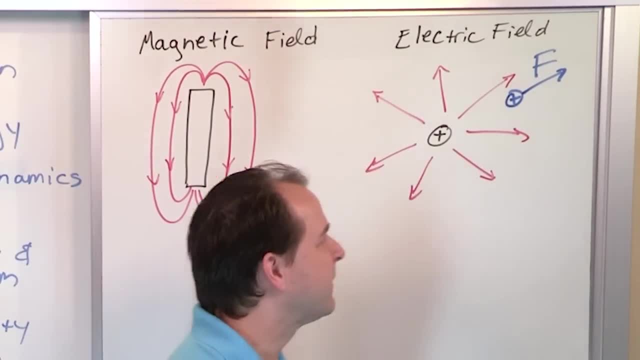 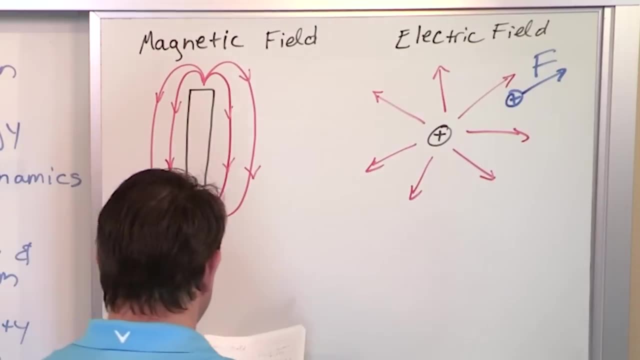 proton with a force F And we're going to learn how to calculate that. And then if you go in here with the magnetic field, interestingly and fascinating from my point of view, if I were to take the same proton and put it inside of this magnetic field and if I just have a stationary 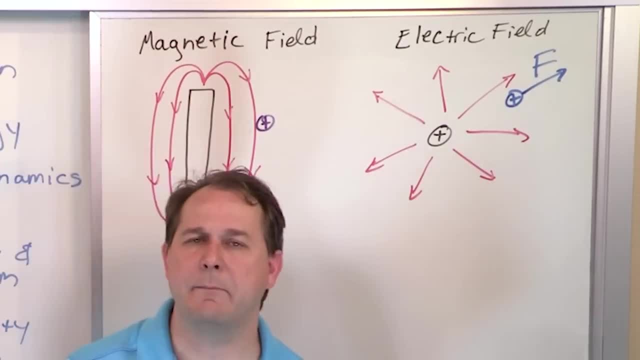 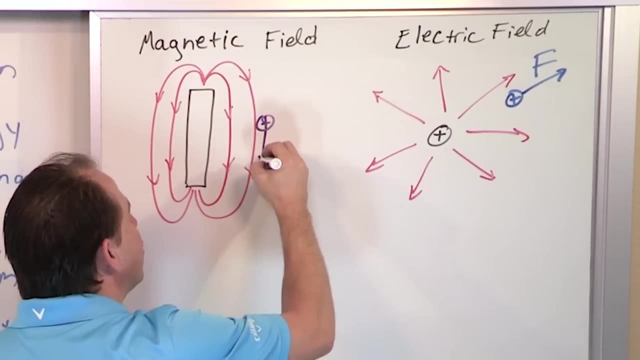 particle here inside the magnetic field, nothing at all is going to happen. The magnetic field will not push on that particle. But if I have this particle, if I start to move this particle myself in some kind of direction, whether it's this way or whether it's this way or whatever, if I start 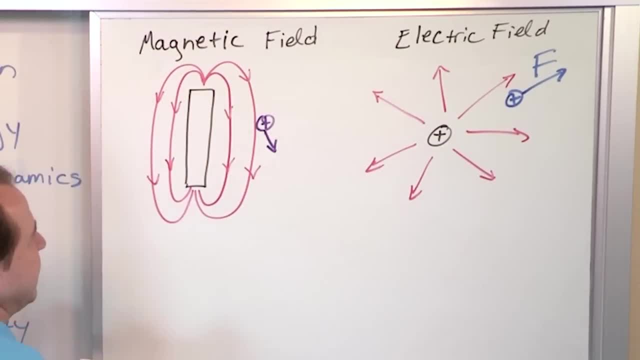 moving it in motion inside of this magnetic field, then a force will pop up and push that particle. The magnetic force will push that particle, but it will not push it along the direction of motion like this one. It'll push it sideways. So it's really bizarre. Not only are the fields, they look different. 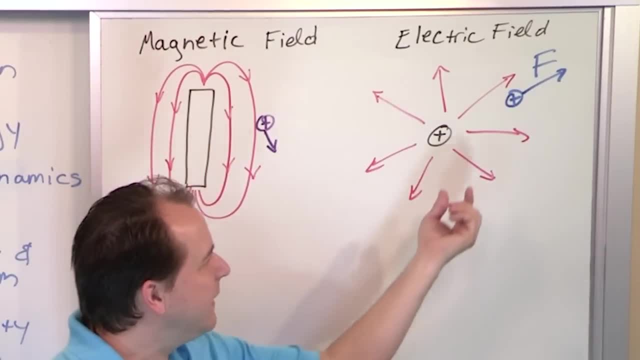 but they actually push on charged particles differently. The proton is pushed away in the same direction of the field lines And the other guy only when it's moving is pushed kind of tangential to the magnetic field right, But only when it's moving, When it's stationary. 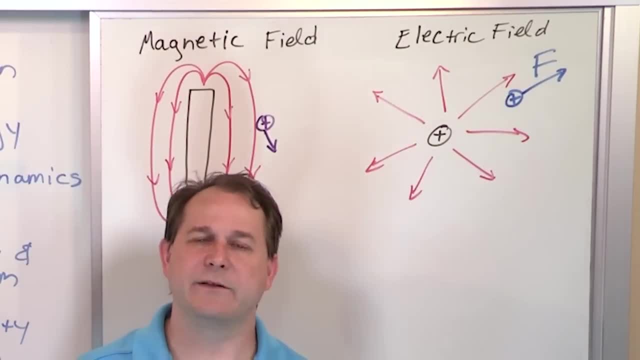 nothing happens at all. So we know they're similar, electricity and magnetism- but they're not quite the same. I should revise that and say that modern physics has combined electricity and magnetism, which seem to be very different things, into a single. 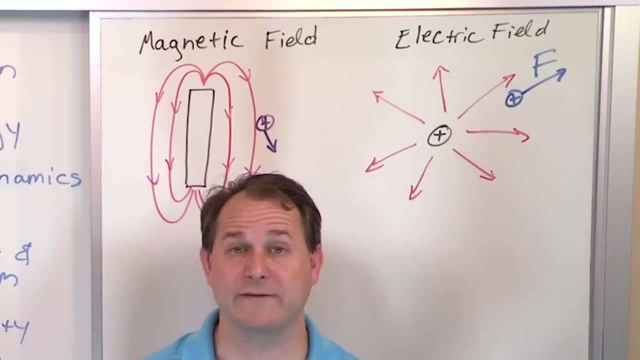 thing called electromagnetism. You may have heard of that- Electromagnetic waves, electromagnetism. It turns out that if you take an electric field and a magnetic field and you oscillate them, then in an oscillating fashion, like we talked about the water waves, then what? 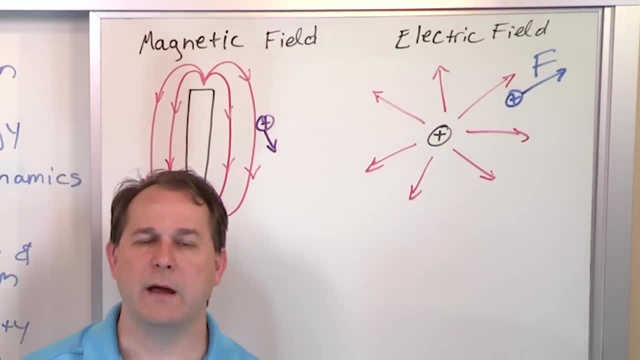 will happen is an electromagnetic wave will form. It'll be oscillating in the electric field and it'll also be oscillating in the magnetic field and it will propagate just like that water wave throughout space. But it'll even go through a vacuum throughout deep space, with nothing there. It'll just travel by. 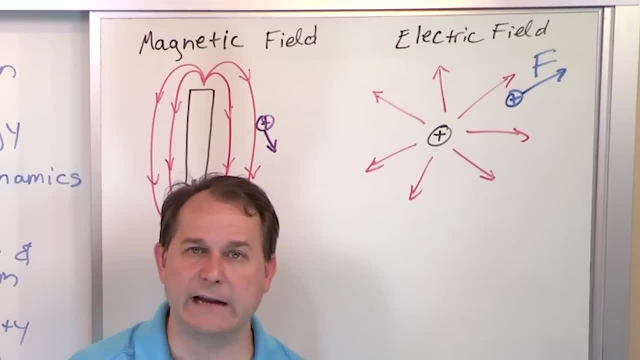 itself and it carries energy. That's how you get a sunburn: It hits your skin and it carries energy from the sun. So why do we care about electromagnetic waves? Well, because you're bathed in it every single day. The light you see now is visible light. Also, we have x-rays, gamma rays, infrared light. 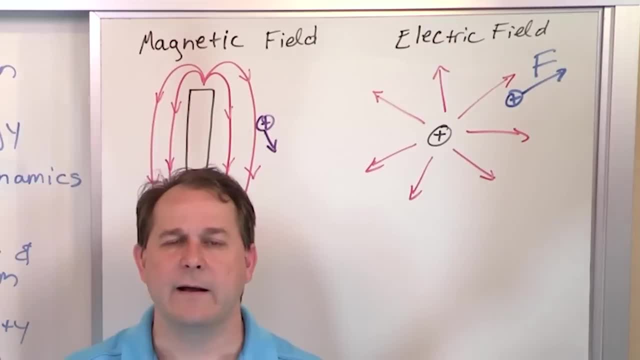 I could go on and on. Basically, all of those are electromagnetic waves. It's just that they're oscillating at different speeds. So it's not just the light that's oscillating, It's the light that's oscillating at different speeds or frequencies we call it. So visible light is a tiny, tiny, tiny. 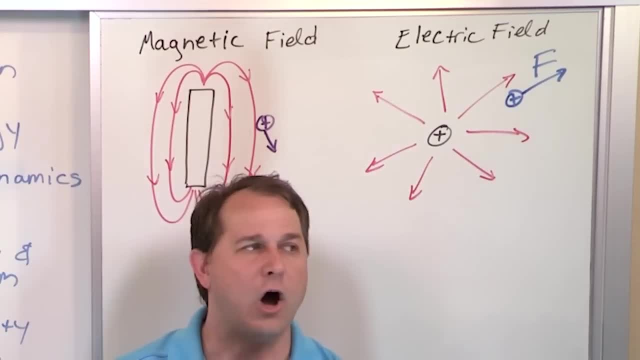 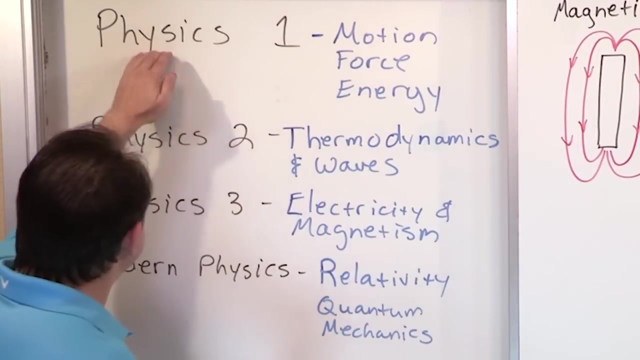 portion of electromagnetism that you can actually see with your eyes. All the other stuff is exactly the same, but oscillating in a region of frequency that you can't see because your eyes just aren't sensitive to it. But it's the same physics involved. So now we've covered physics one, physics two. 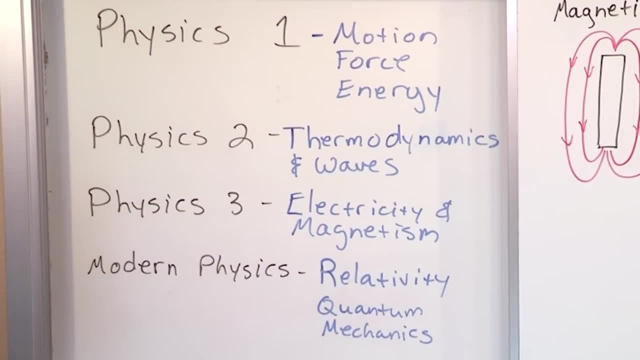 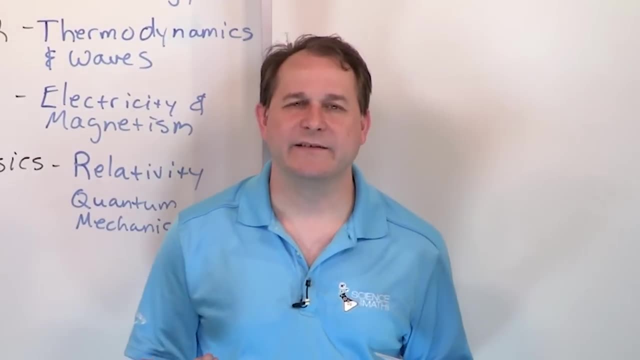 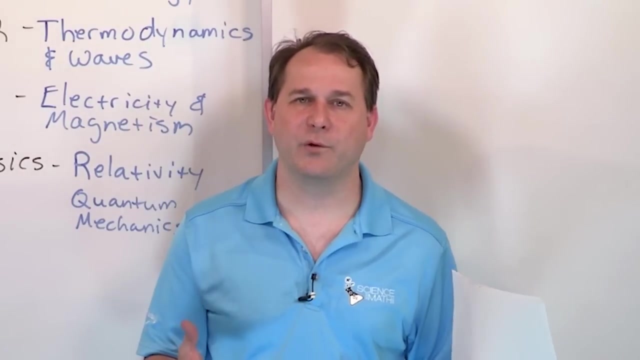 physics three overview. and next we're going to talk briefly about one of my favorite things: relativity and quantum mechanics. Now, truthfully, you're living in an amazing time, because you can open up a book or watch a lesson or get a lecture from knowledge that was handed down before you about some of the craziest. 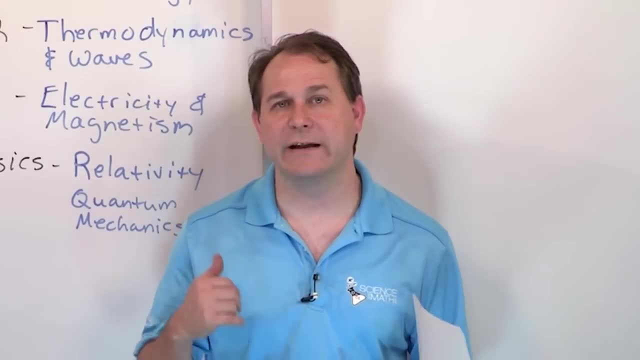 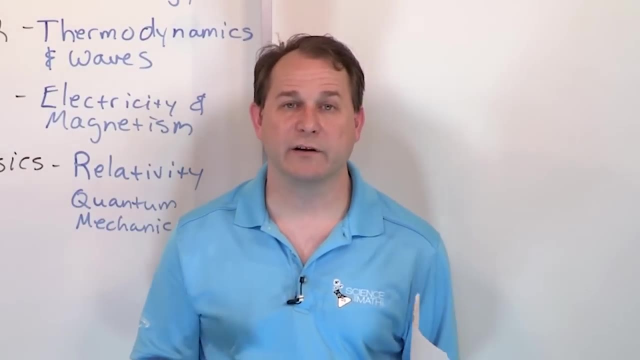 wackiest stuff that we've discovered to be absolutely true about our universe, and that's relativity, Einstein's theory of relativity, and quantum mechanics, which was developed by many people. Both of these theories were done in the early part of the 20th century, so about 100 years. 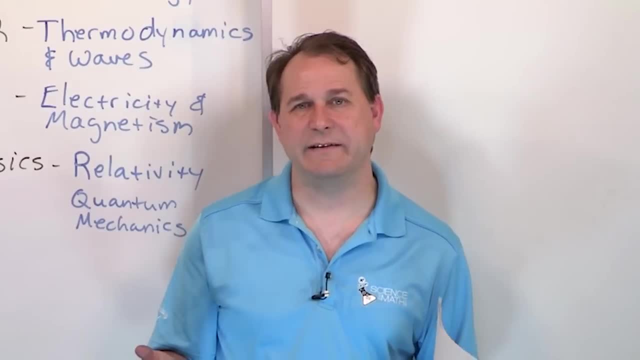 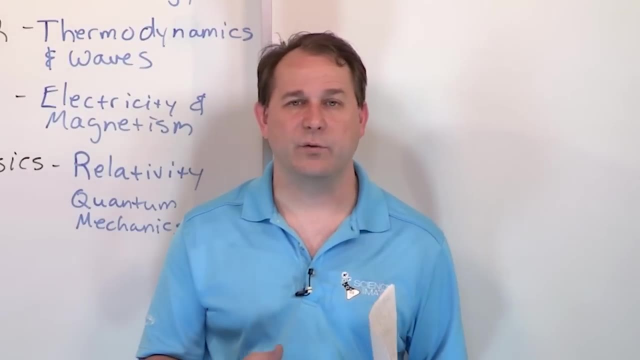 old And, to be honest with you, we still don't quite understand these theories Totally. I mean, we understand a lot about relativity. We don't understand quantum mechanics that well even today, And there's tons of problems, real problems, that we can't solve in either. 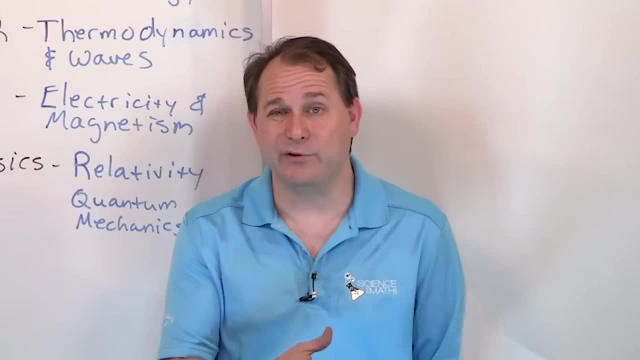 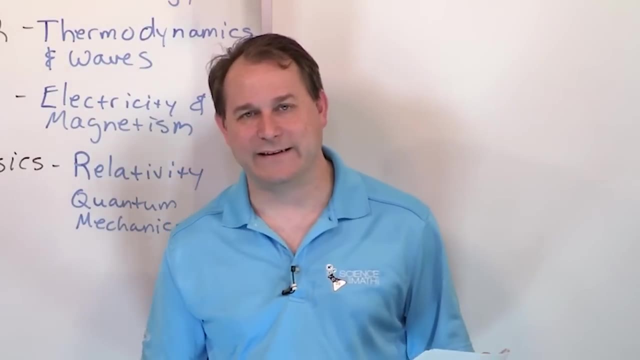 theory just because the math is too hard. But we understand how we would do it. we just the math gets so difficult sometimes. But the basic idea about relativity I talked to you about before is that time and space- I didn't mention the space before time and space- are relative to your state. 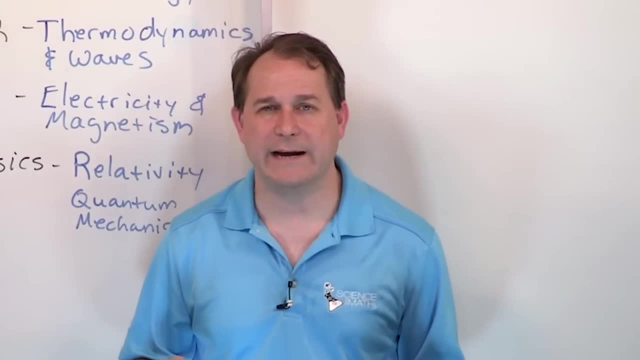 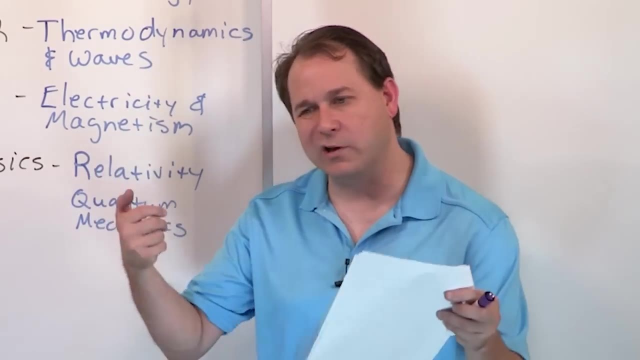 of motion. If I move really fast, near the speed of light, time and space are relative to your state of motion. Time and space will behave differently for me than it does for you if you're not moving. And that seems weird because if I take two clocks and they're synchronized, tick, tick and they're both. 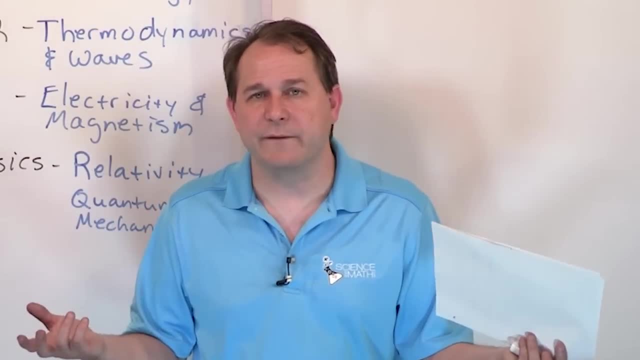 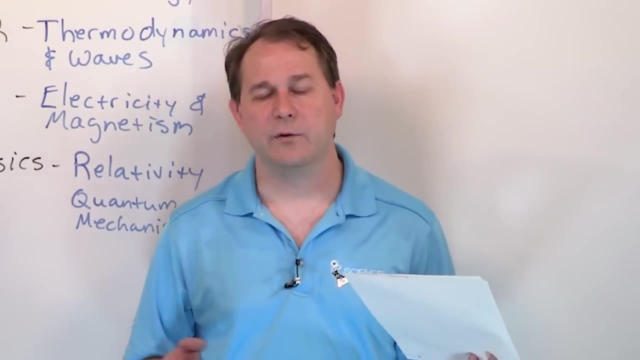 the same, you think that time would exist, the same for both of us. That's our everyday experience. But in fact, if you actually go fly that second clock in a spaceship and get really close to the speed of light- which we can't do- but if you could do it, then when it came back you would 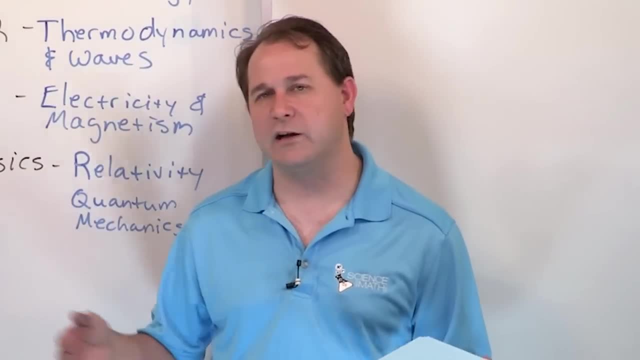 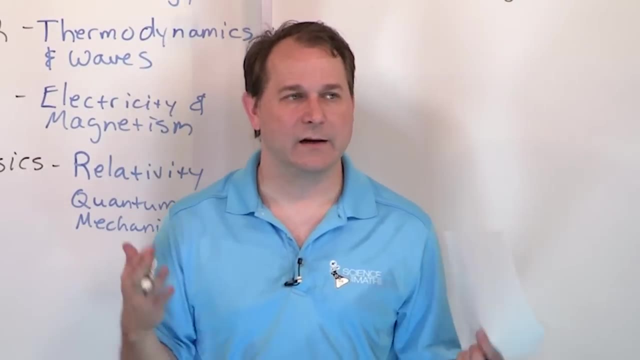 find that that clock has a different time elapsed than the clock on home at home. How close. Well, we have to do some problems to illustrate that. But when I say how close, I'm talking like .99999 times the speed of light, which is incredibly fast, because the speed of light 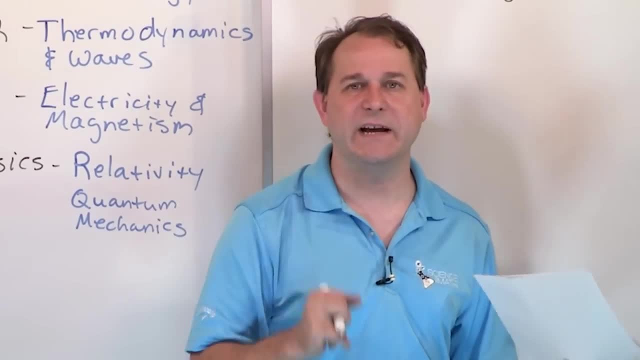 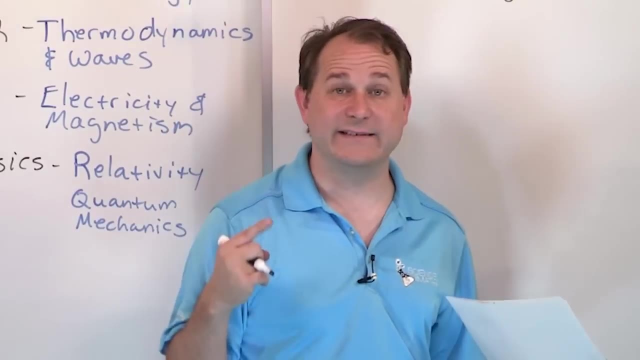 can go seven times around the planet Earth in one second. So think about that's one second, that's another second, that's another second. Every one of those seconds, light goes around the planet seven times. It's incredibly, unfathomably fast. So, to be honest with you, 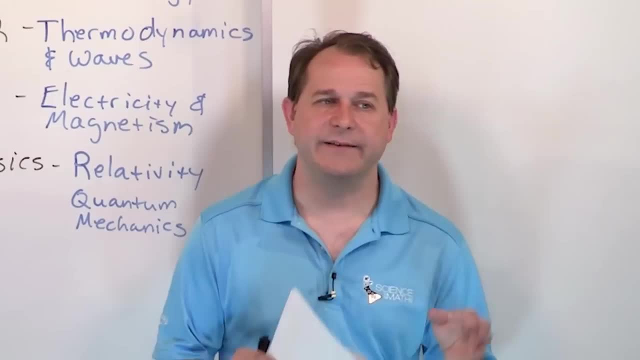 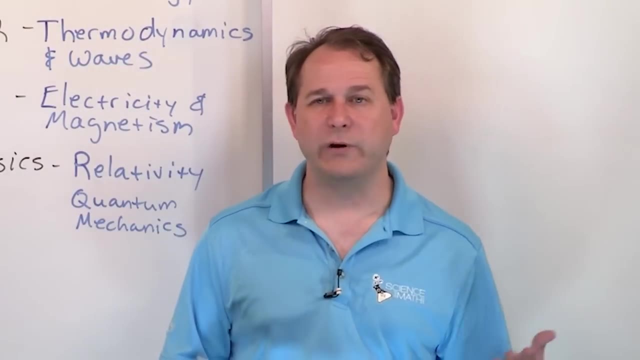 wrapping your brain about the idea around. the idea that time can be different for two people depending on their state of motion, how fast they're going, is very, very hard to accept, because we don't see it every day And the reason we don't see it is because we don't travel very fast. We're traveling at a snail's pace. But we've proven that these things are true by looking at accelerating electrons and other particles in particle accelerators, because we can get electrons going very close to the speed. 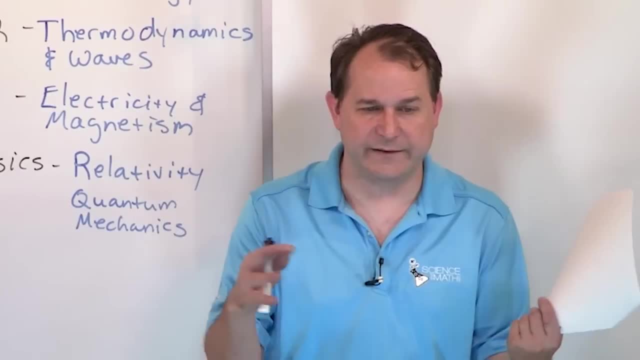 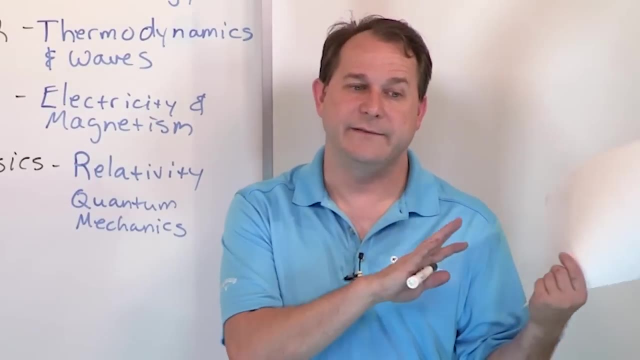 of light. We can get other particles that exist that are going very near the speed of light, And we can. it's a long story with the way the experiment, the science are done, but we can definitely show that time travels differently for different people. We've actually taken atomic clocks- very accurate clocks- and flown them on airplanes- It's not near the speed of light, but it's as fast as we can go- And we get those clocks and we compare them when we come back down to Earth and we see that the clocks don't. 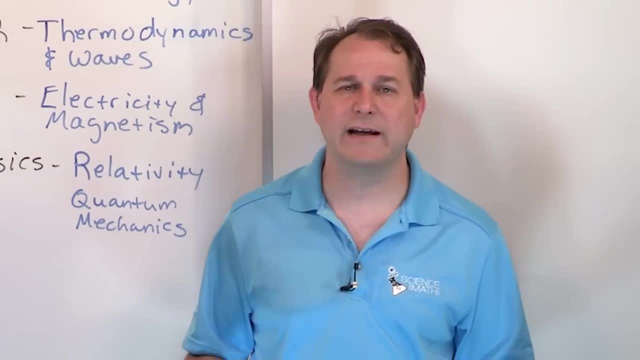 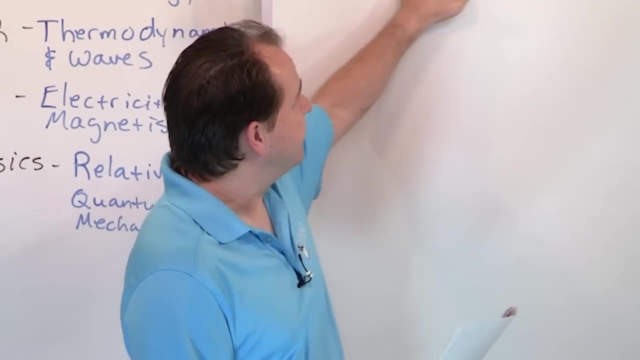 agree anymore, Because time actually it wasn't because the clock is broken, it's because time actually ticks differently depending on how fast you're moving. Now the second part of kind of modern physics, and I'm going to talk a little bit more about that in a 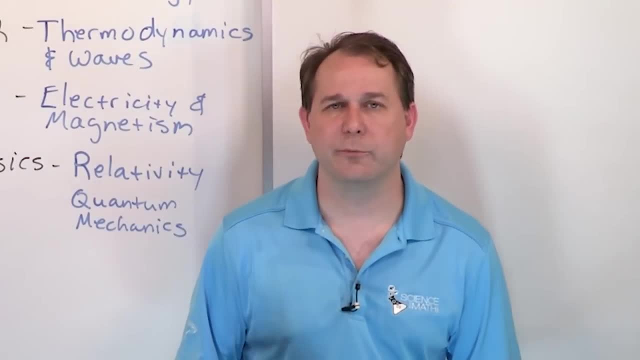 minute is quantum mechanics. There's a lot to it, but we call it quantum mechanics And I know that you've heard that term, but it's a nebulous, scary sounding thing And, to be truthful, as I said before, nobody really understands why quantum mechanics works. the 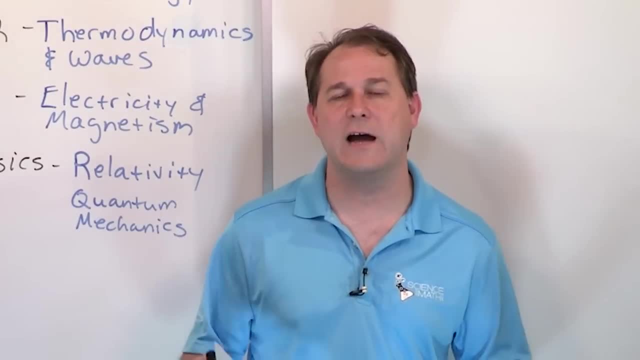 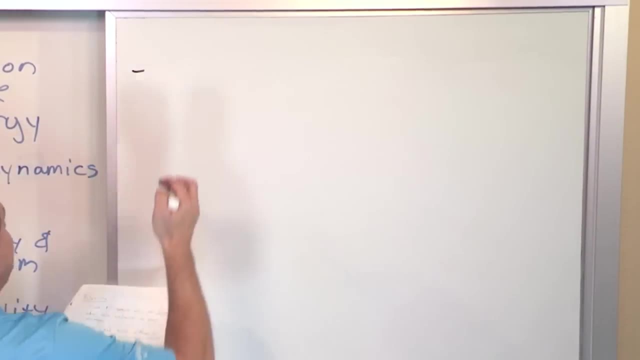 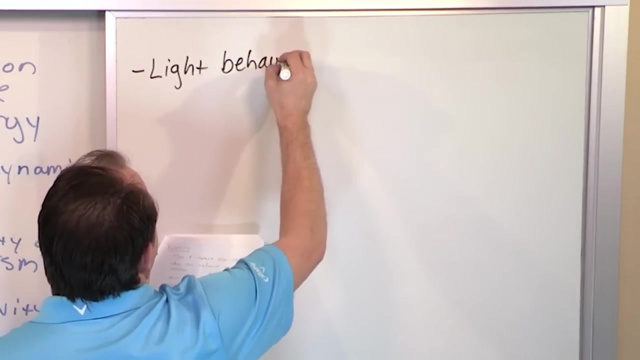 way it does. But what we do know is that it absolutely does describe our reality. So one thing we know: remember I told you light was an electromagnetic wave. Well, it turns out that light, when you actually do detailed experiments on it, it behaves as a wave in. 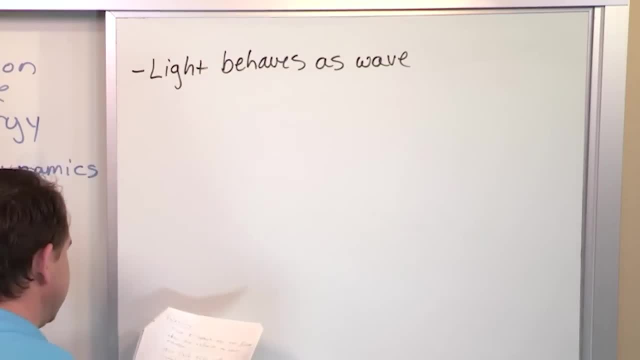 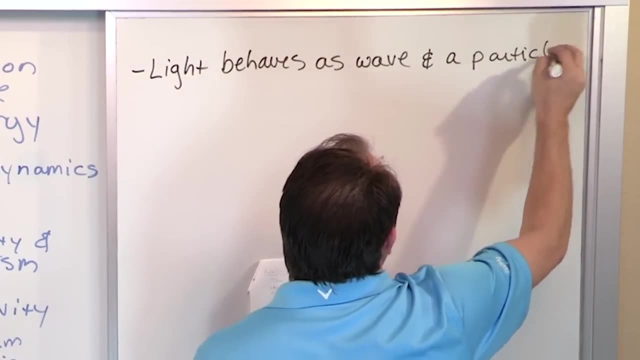 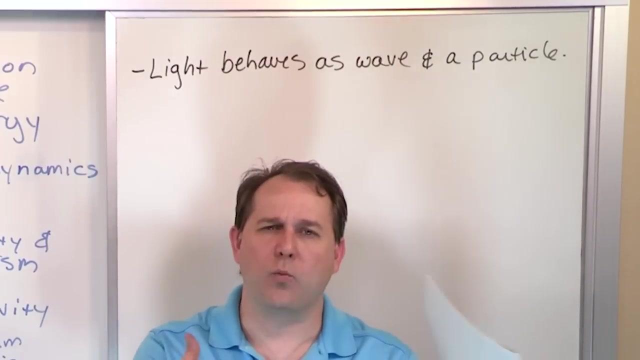 some experiments, like we talked about oscillating electromagnetic fields, And it also behaves as a particle. The particle is called a photon, So I know you've heard the term photon, photon of light. Well, in some experiments light can behave like a wave and we'll get into 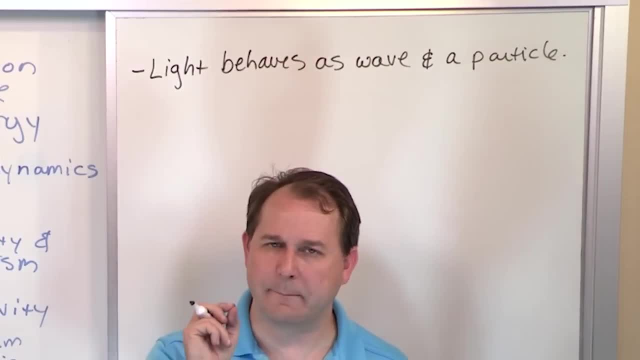 the details later, But in other experiments it behaves very much like a particle, like a. I don't want to call it a solid object, but a discrete object called a photon. So is it a wave or is it a particle? Well, truth is it's both. 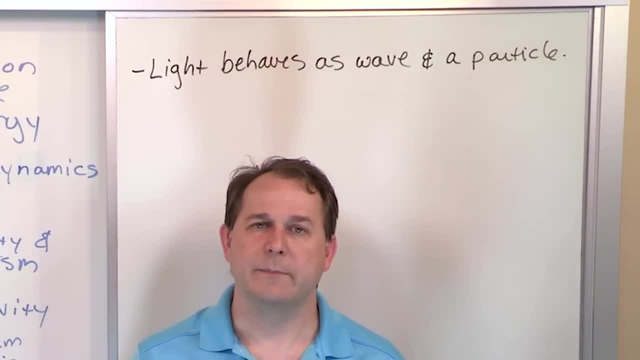 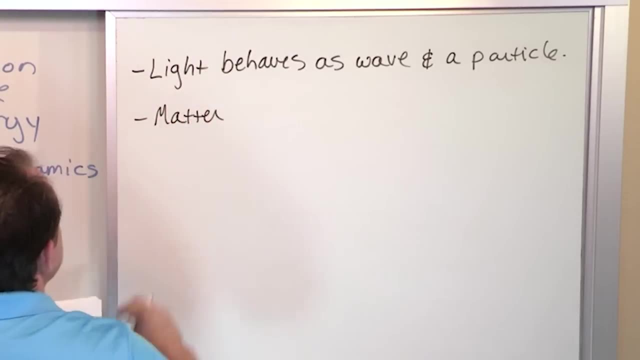 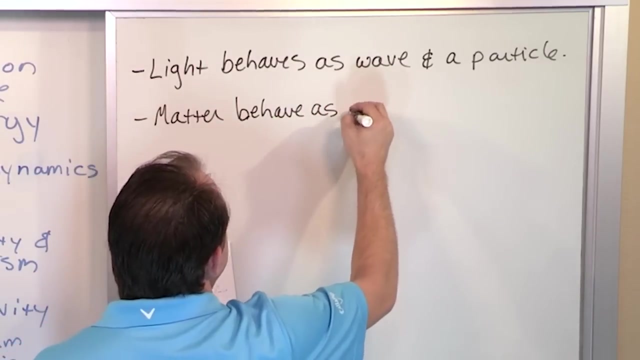 It's something else that we don't have a word for. that's called a wave and a particle. Now here's the other part that will blow your mind. Matter meaning electrons, protons, pretty much anything can behave, obviously, as a particle, because we've done lots of experiments. 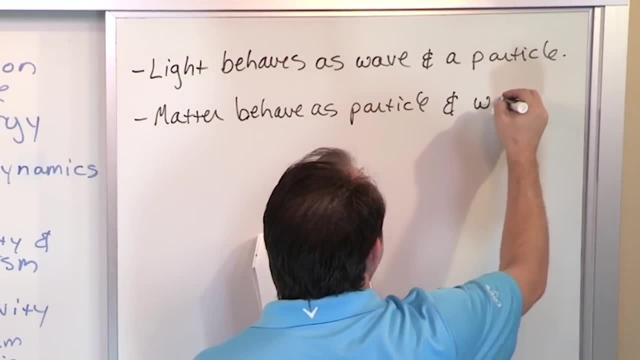 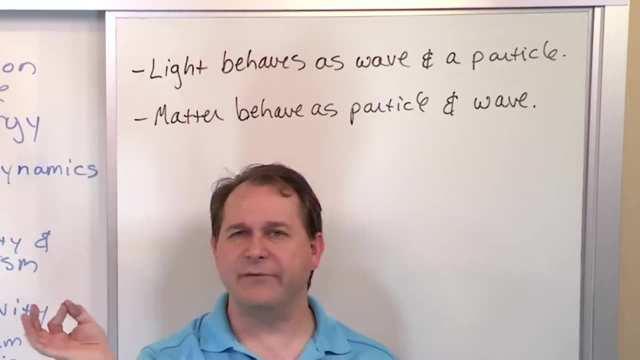 with electrons. We know they're little particle things, but it can also have characteristics of a wave. That should blow your mind, because it's absolutely crazy that I can take an electron and it can behave in some experiments like a little discrete particle, but in other experiments 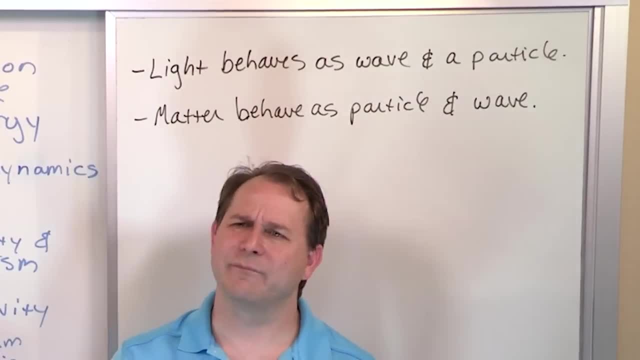 it can interfere, like waves interfere. So are electrons particles or waves? Is photons particles or waves? Well, it turns out that when you really zoom in to the microscopic level of our reality, a different set of rules apply. Actually, all the same rules are applying all the time. 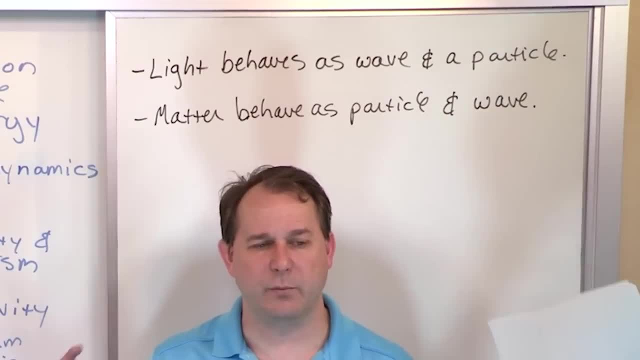 but they just manifest differently at these large, large scales that we live in. But when you zoom in, you can see the rules for what they really are, and photons and electrons and protons, they all have different characteristics. So what we're going to do is we're going to 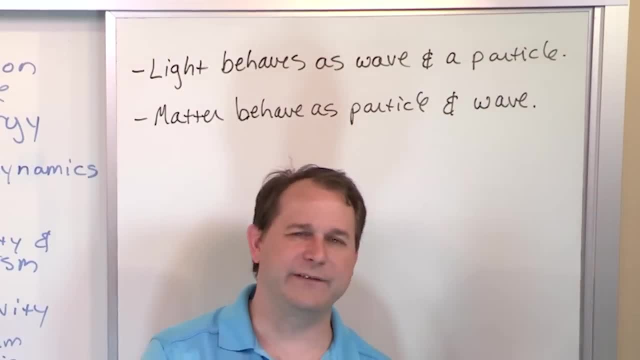 look at them one by one. They all behave what we call quantum mechanically. They have characteristics of a particle and also characteristics of a wave. What are they? Who knows? We can't really see them, We can't touch them, We can't poke them with a pair of tweezers, but we 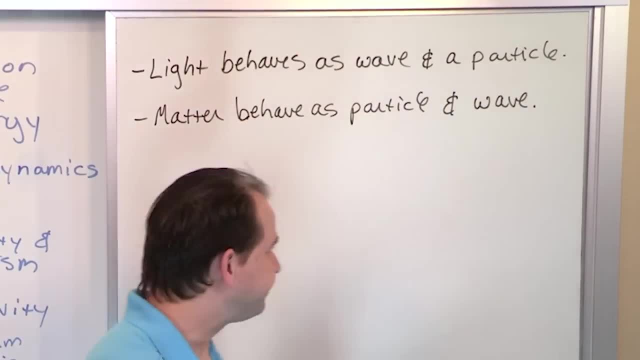 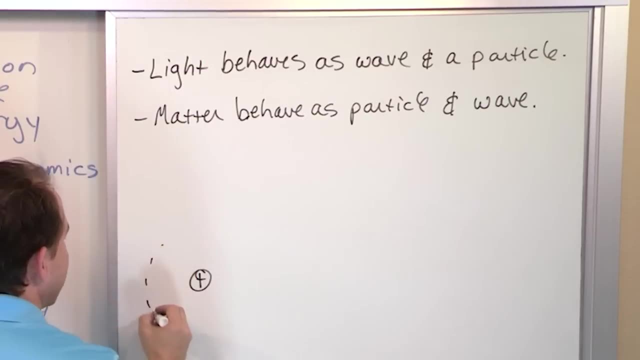 can do experiments and we know that they behave with these different characteristics. What we also figured out with quantum mechanics is that if you have a proton and a nucleus of an atom, right that the electrons. you probably already learned in kind of chemistry. 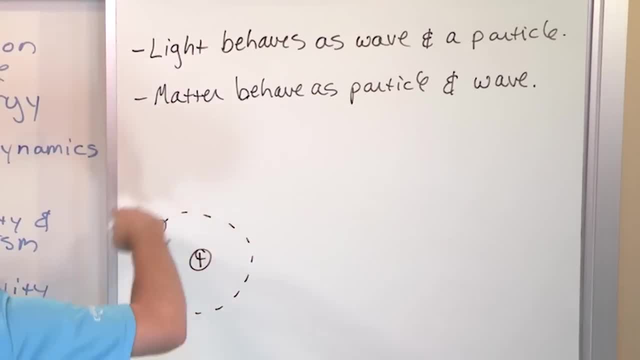 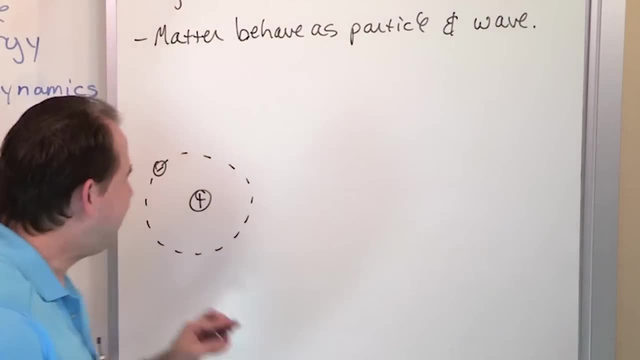 class that you might have, like an electron, like right there, and we say it's going around the nucleus. Well, it turns out it doesn't really behave like a solar system going around and around and around. We'll get into the details later, But these electrons they can. 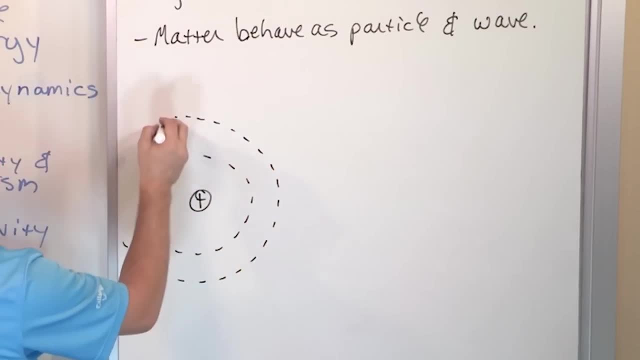 only exist in what we call certain energy levels. So this might be energy level number one and this might be energy level number two. The electron can never, ever, ever ever exist in between these energy levels, which is weird, because the moon or satellites in 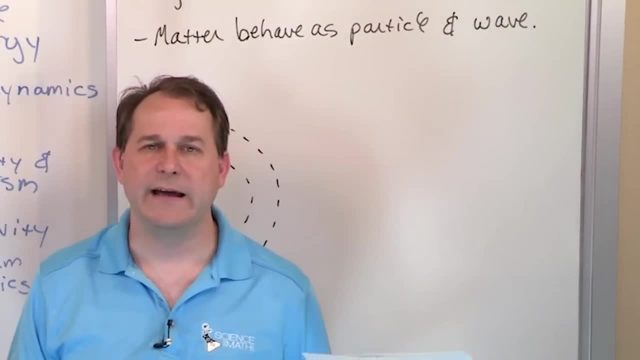 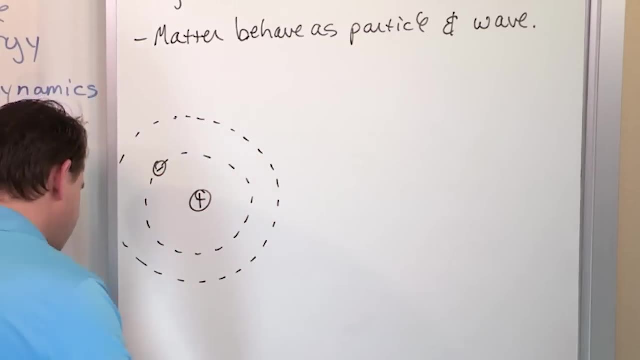 space. they're going around the Earth. We can put a satellite anywhere we want in the Earth's gravity field, but you cannot put an electron here in between the energy levels. Right, It has to be in discrete energy levels. But what you can do is I can put some electricity. 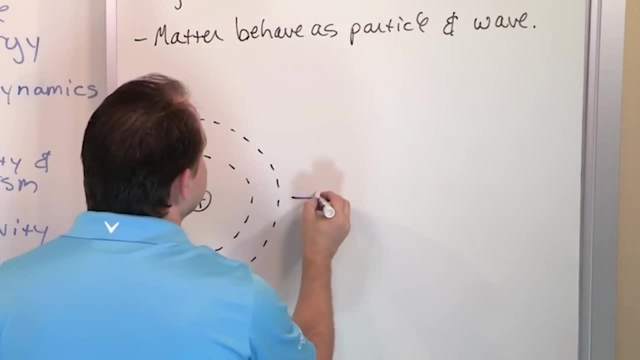 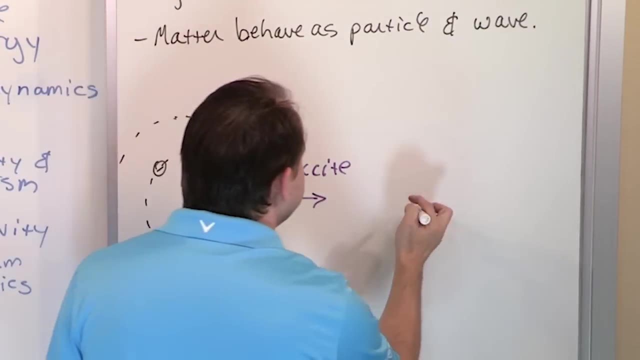 into this and I can pump this electron up into the higher state So I can excite it. I can excite it, maybe, with electricity. So what happens when I do that? Well then I'm going to have the proton in the same place. I'm going to have energy level number one. 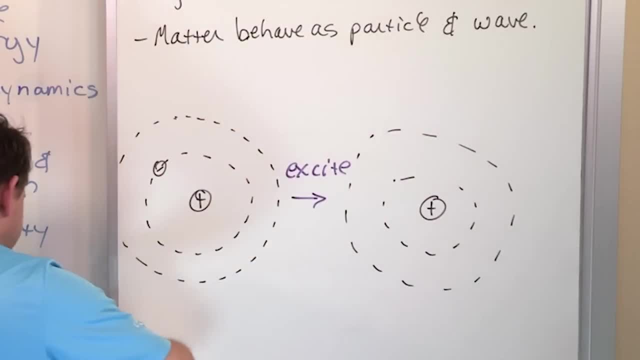 I'm going to have energy level number two And the electron, when I excite it with electricity, is going to move from this guy. It's going to pop up temporarily up to the higher energy state, But it's not going to stay there forever. As soon as I stop exciting it, it's going. 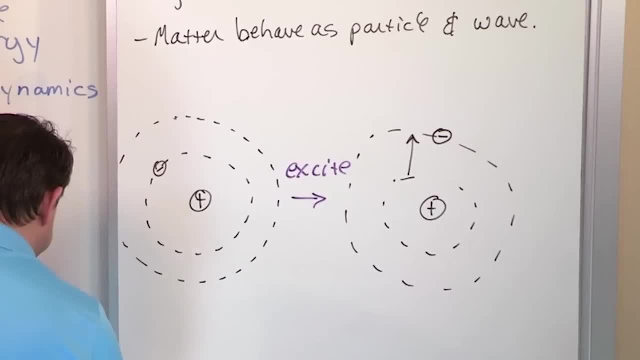 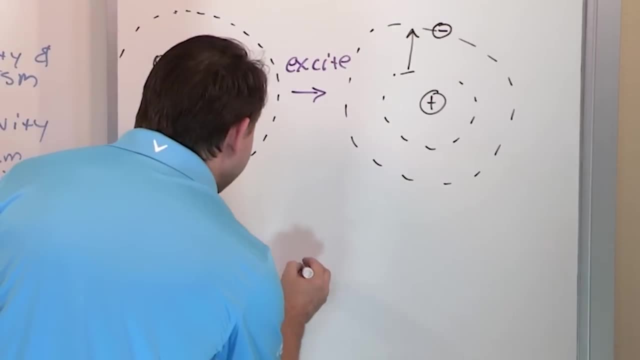 to decay right back down to the lower energy state that it likes to live in. So I'm going to put a little arrow here and I'm going to say it's going to decay. Now, what happens when it decays? That's the interesting part. What's going to happen is you have a proton. 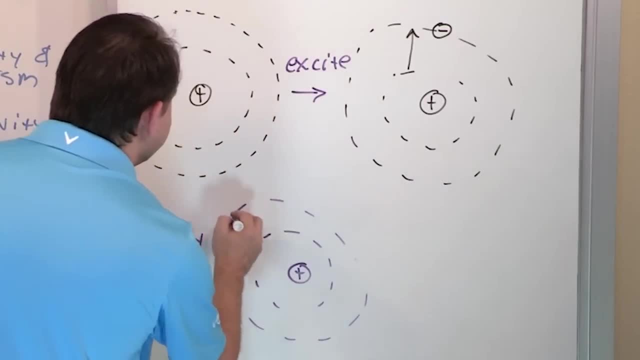 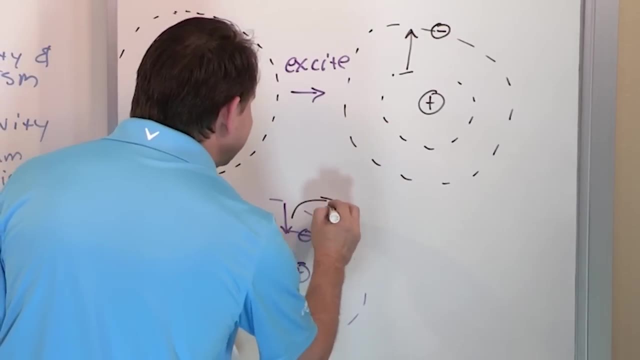 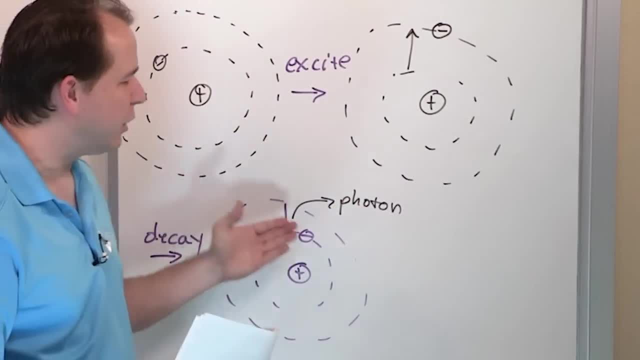 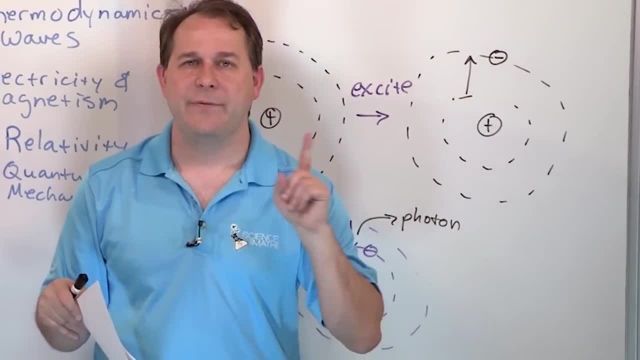 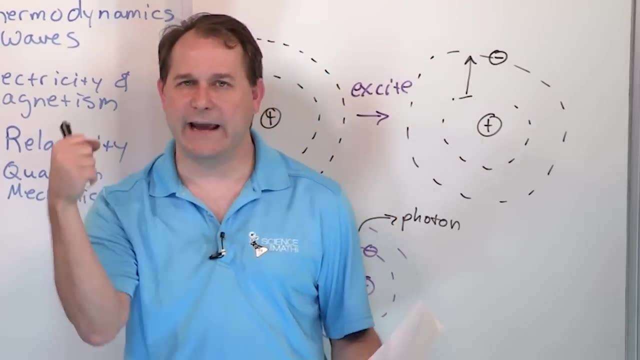 decay back. But when they decay back, they release a photon. That is what is happening when you take a piece of iron and you heat it in a campfire And you pull it out of the campfire and it's red. Why is it red? Have you ever thought about that? Why is it glowing? 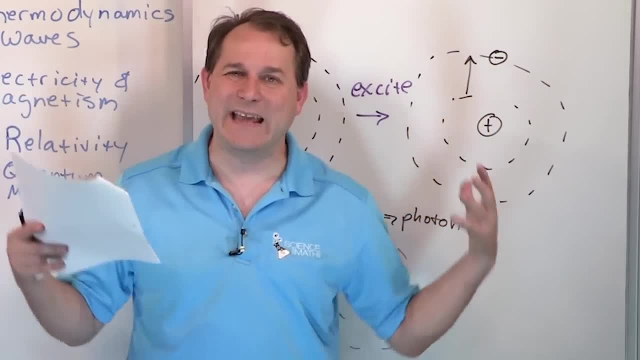 It's because all the electrons have been pumped up from the fire, from the energy, and they're a lot more existing in this higher state. But when I pull it out, I get the heat exists in the air, But when I pull it out they start decaying down. 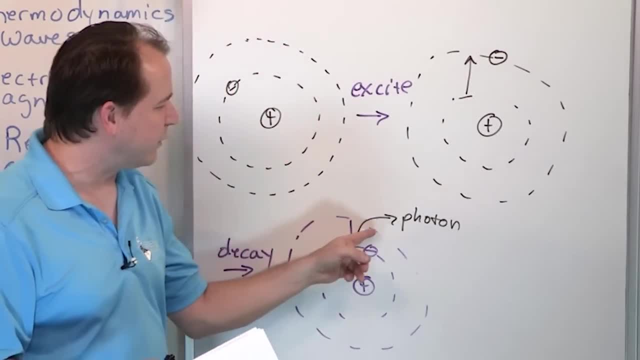 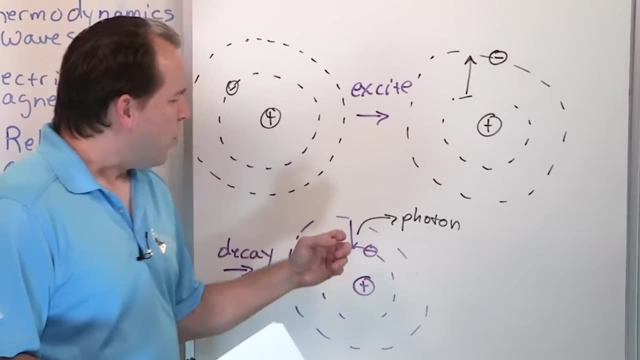 There's billions and billions and billions of them. They start decaying down And when they do, they start releasing photons, which are light, light particles, which we already told you could be a wave or a particle, right? Why do we care about this? 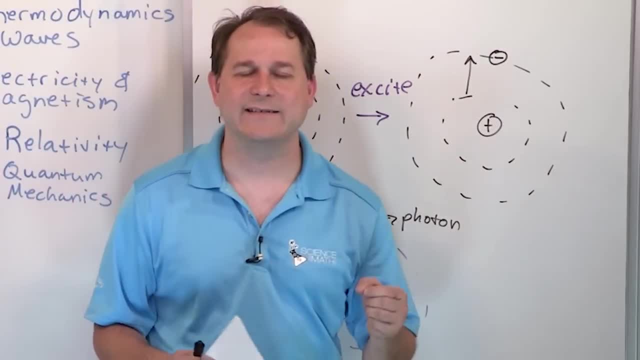 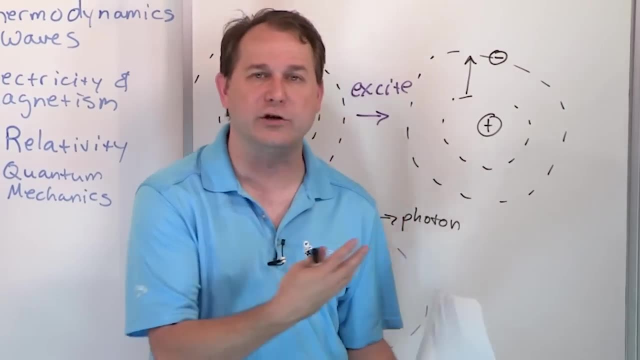 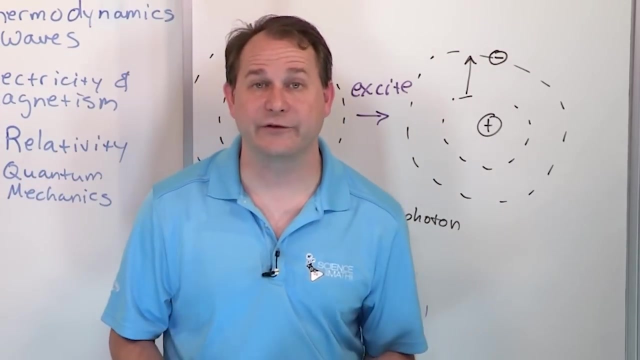 Because we can use matter to make photons. That is how all computer screens are made Like actually screens on your phone. We use these quantum mechanical effects to make those screens. We use these effects of the way energy levels work to make things called transistors, which.